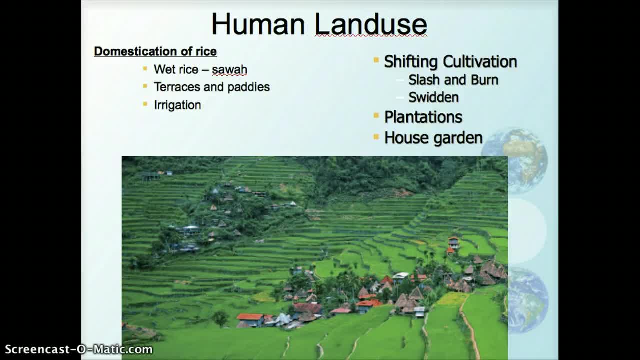 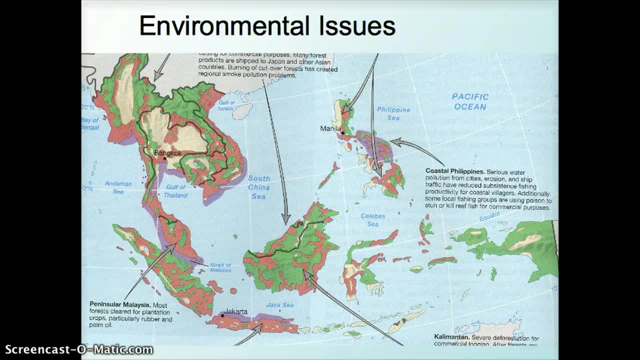 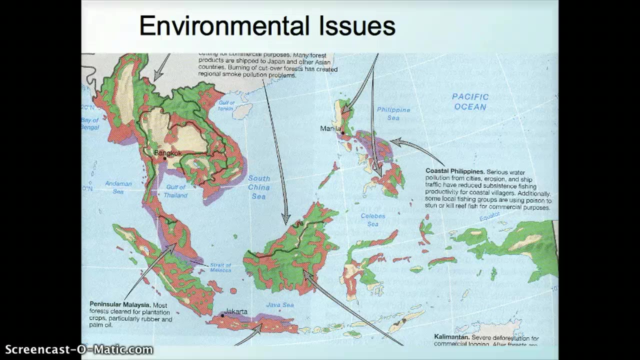 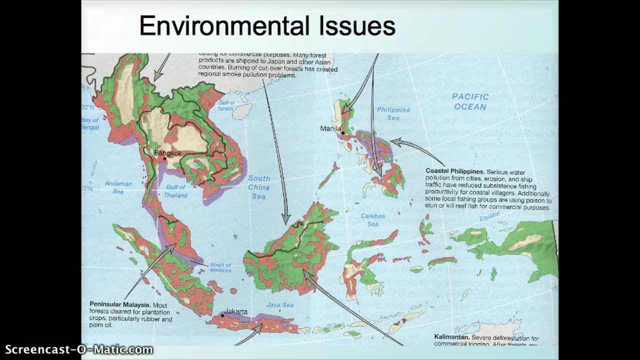 for house gardens, for subsistence. With this increase of plantation-style agriculture and also the extraction of timber, there are a lot of environmental issues that we find throughout Southeast Asia, particularly deforestation in places like peninsular Malaysia and in Indonesia. There's also serious water pollution. 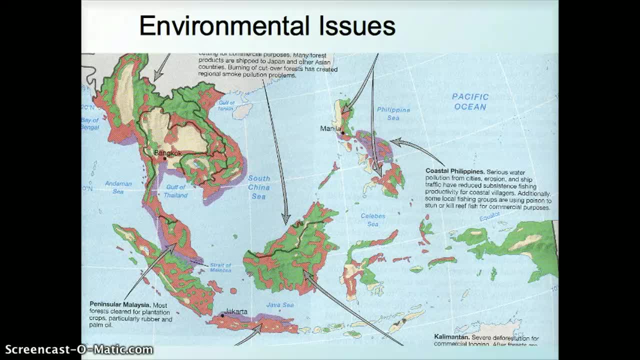 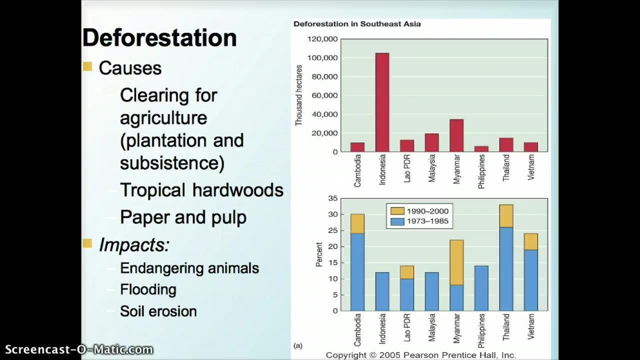 from cities, erosions and ship traffic in places like Indonesia, and this has been especially detrimental for folks who are using the ocean for a lot of fish as a resource. So, looking at some of the causes and consequences of deforestation- again one of those things. 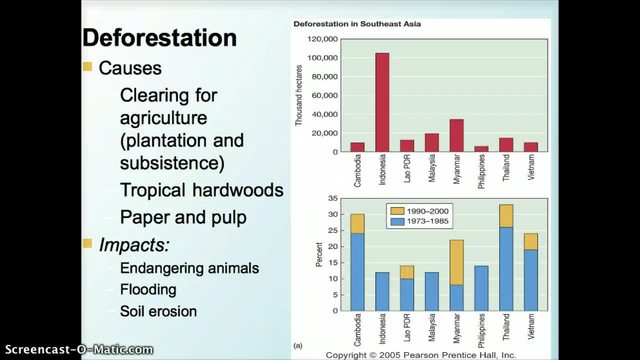 is the clearing of land for agriculture, both for plantation-style export agriculture and subsistence, and the production of tropical hardwoods, paper and pulp. We see with that endangering of major animal species because of a lack or loss of habitat, flooding as. 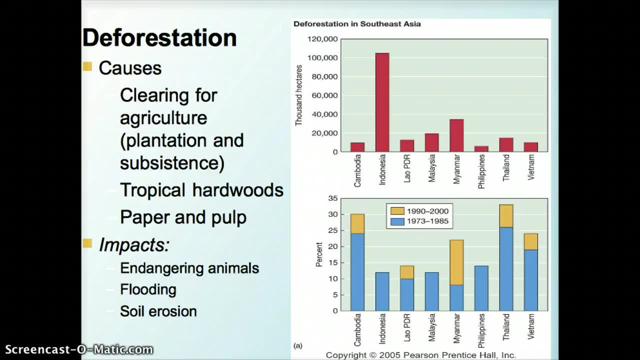 these areas get a lot of rainfall and without the forests there to help hold the soil in place, you're able to have much more runoff and soil erosion. So we see a lot of deforestation and flooding as a result. If we look at how deforestation is distributed across the region, 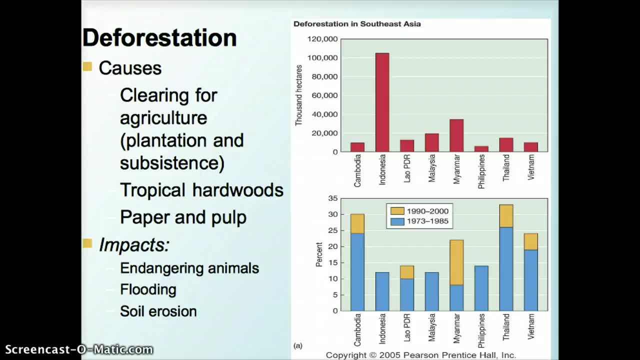 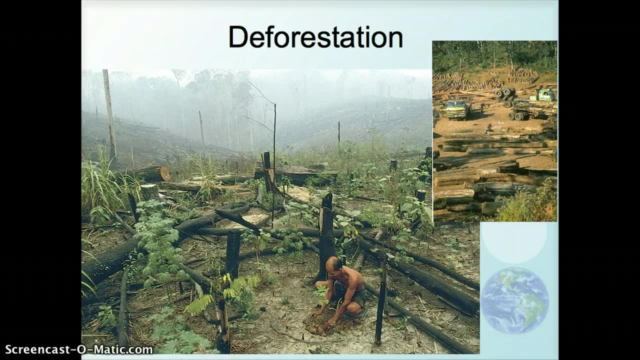 we can see that Indonesia is by far the leader, with over 100,000 hectares having been deforested, Myanmar as well as also having major deforestation there. Here's an example of some of the types of landscapes left after the deforestation process. 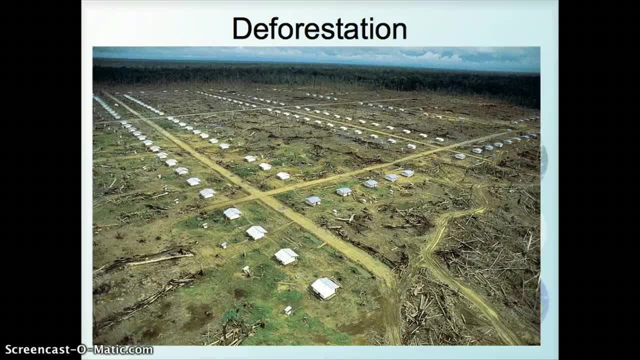 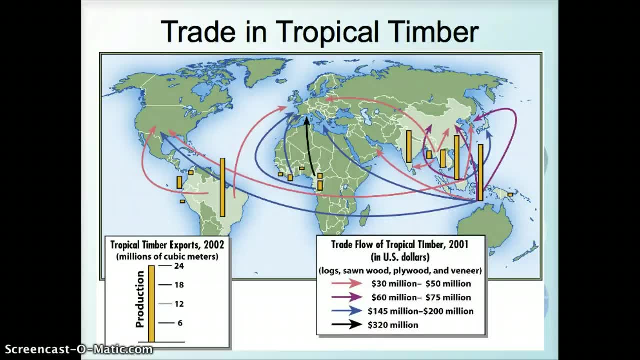 In areas that have been cleared for new housing developments. It's important to not only think about these places as sources for tropical timber, but also to think about where the flows of these goods go, And we see that a lot of these exports travel to places within eastern and southern Asia, So you can see a majority of these areas. 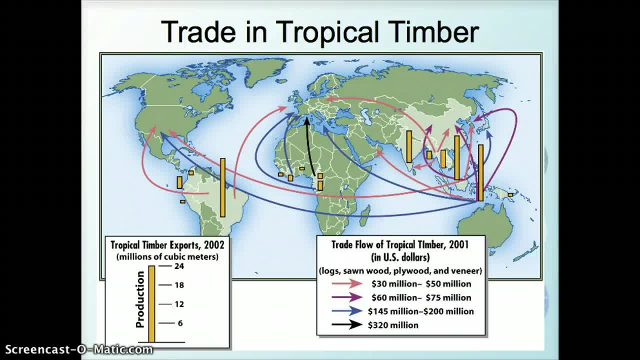 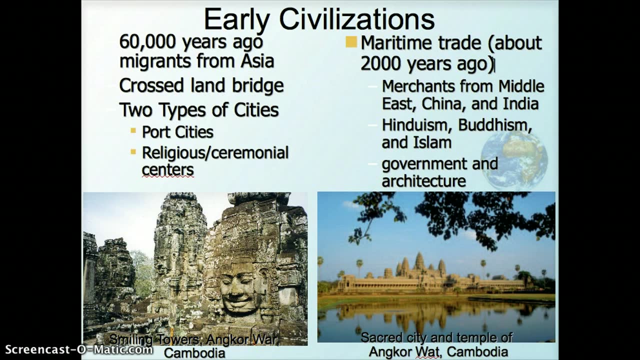 are coming from the lower reaches of Asia, but we also see a majority of exports coming from Indonesia, going to places like Japan and China as well. We mentioned earlier one of the aspects of Southeast Asia as being a sort of crossroads for a lot of different cultures. So around 60,000 years ago, migrants came from the continent. 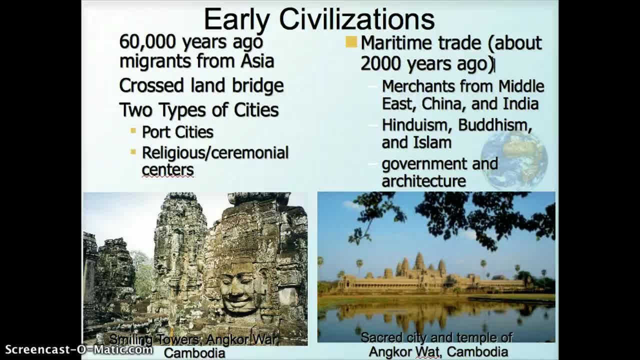 a land bridge that existed at the time and peopled, uh, this area at the time. there was then two types of cities that emerged: port cities for trade and religious and ceremonial centers. you still see kind of a focus on dual cities within many of the countries in southeast asia either, because 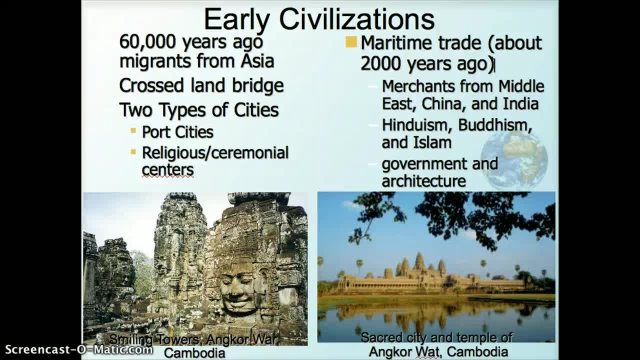 of this tradition or things like conflict. so, for example, in vietnam- vietnam having been split between north and south vietnam for a time- you have two major sort of cities there as well, so in a lot of places you have these dual city systems. maritime trade was a major influence. 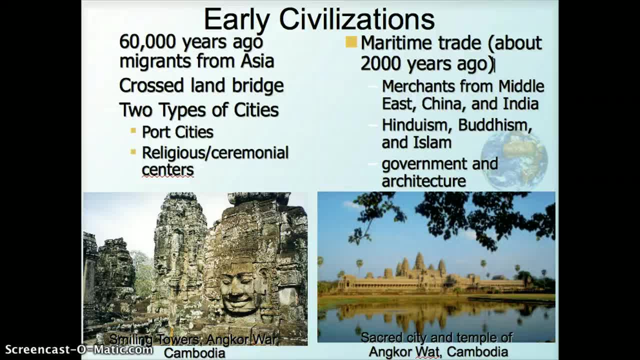 beginning about 2 000 years ago, and so you had merchants from the middle east, china and india all traveling through this area for trade, and so you have a tremendous amount of religious and cultural diversity where hinduism, buddhism and islam are all present. 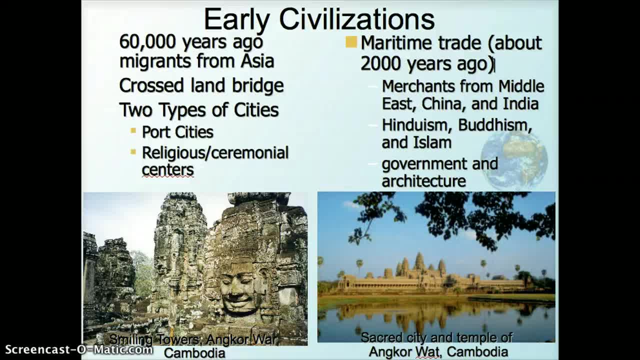 in terms of religions, in terms of government, society and architecture, and you see that sort of combination in some of the aspects of southeast asian culture. some of these images below show um, one of the major uh sort of religious ceremonial centers in krawat in cambodia. 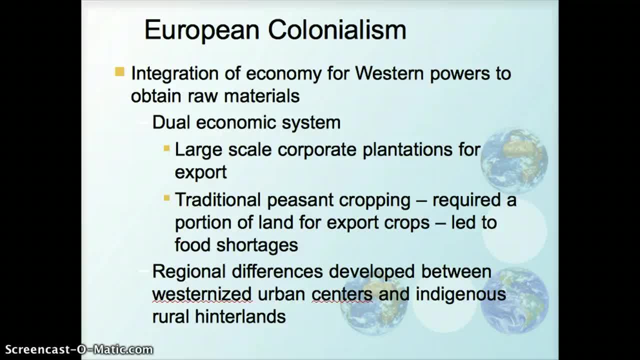 with european colonialism you saw an integration of this area in into the world's economic system and kind of a dual economy that emerged. european colonizers were interested in trying to set up large-scale corporate agriculture on plantations for export, and so you had that sort of as a reorientating of 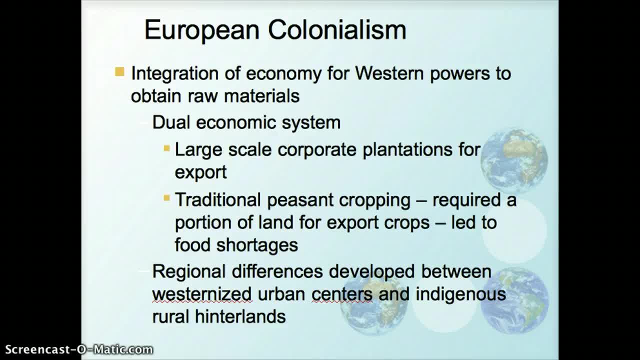 local systems of production, but then you also had traditional peasant cropping that existed, and a portion of land was left for that to be used for agriculture, and so you had a lot of that, but it was a very diminished portion of land, which often led to food food shortages. you also 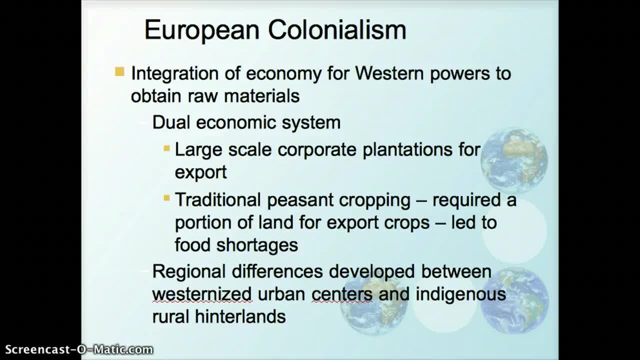 see the development of a real differentiation between the urban centers and the port cities that had a lot of contact with european colonialization and the world economy, and indigenous and rural hinterlands. so you have a sort of dualism within the countries themselves. some of the major 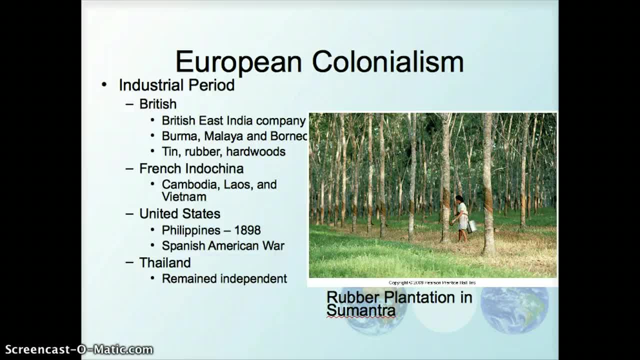 areas within this and during, of course, this period of industrialization and the industrial revolution in europe were britain- you see the british east india company expanding and especially interested in growing rubber implantations for tin and hardwoods in indochina. or peninsular southeast asia- you have the french having holdings in cambodia, laos and vietnam. 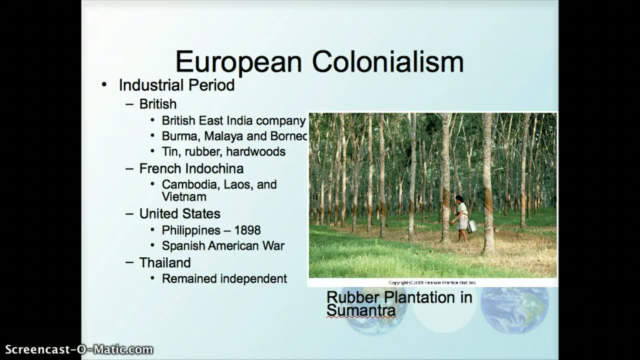 later the united states becomes interested in this area after the spanish-american war, has the philippines as a colony and thailand was an area that remained independent. here, of course, the us also became involved later in the 1960s as the french left vietnam, and there was a conflict between the communist north and southern vietnam and the. 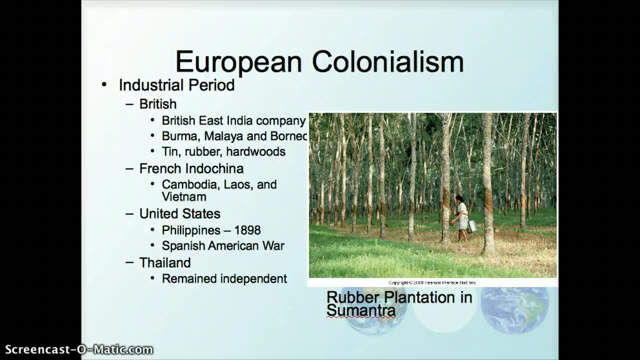 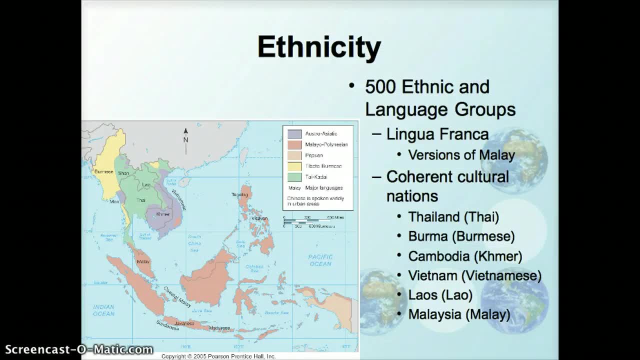 us entered into that conflict there as well. if we look at the culture within this region, there is a lot of diversity. for the country there are 500 different ethnic and language groups. many are related to the lingua franca of melee or malaysian. there's many coherent nations in terms of culture, so a sort of overlap between. 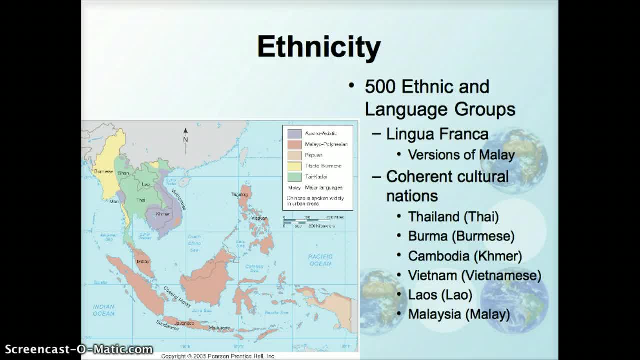 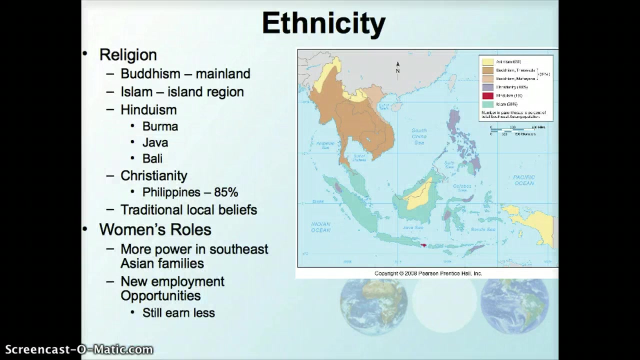 the idea of a nation and a state. so, for example, the people in thailand being majority, identifying with being thai, vietnam, vietnamese, etc. if we break down ethnicity a little bit farther, we can see that, in terms of religion, we have buddhism as being the dominant religion on peninsular southeast asia. 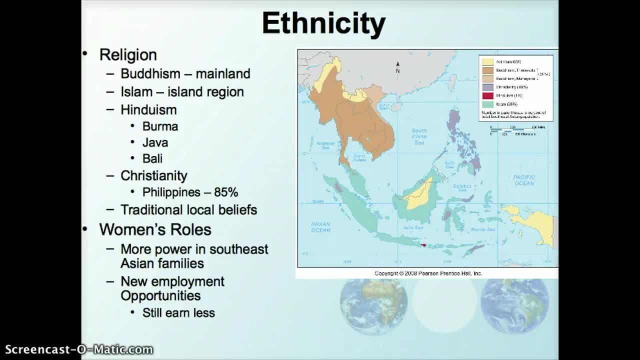 in the island section, particularly indonesia, islam is the majority religion. indonesia is actually the most most populous islamic country in the world. you also have hinduism in burma, java and bali and christianity in the philippines. from that legacy of spanish colonialism and catholicism there's also a lot of sort of integration between traditional 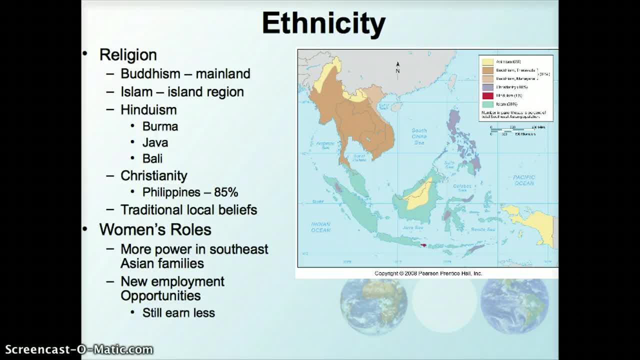 local beliefs and these larger sort of world religions. southeast asia is really interesting too in terms of women's roles. so women in southeast asian families tend to have more power within the family itself, so somewhat less patriarchal in terms of the power structure within the family. and then there's been a lot of new employment opportunities for women with the new industrial. 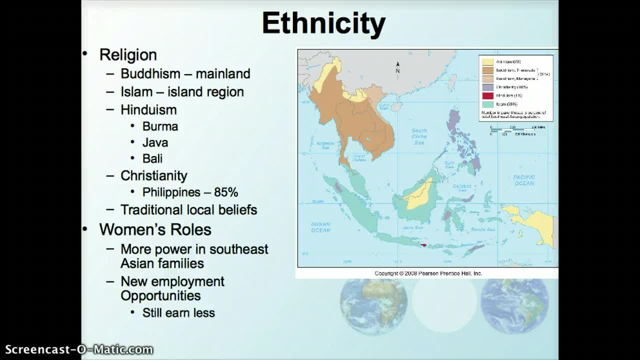 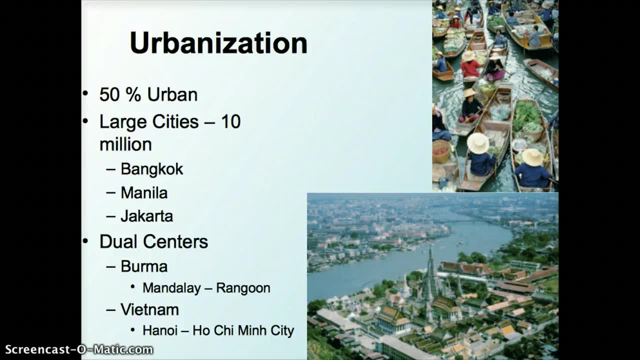 division of labor, but still women often earn less. so the area is about 50 urbanized, with many large cities that have over 10 million people. so places like bangkok in thailand, manila in the philippines and jakarta in indonesia- again you see those dual centers in places like burma. 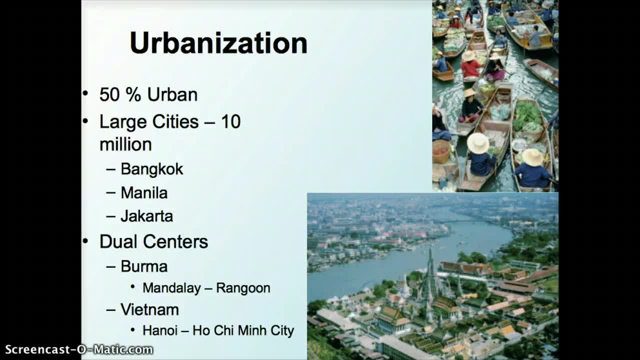 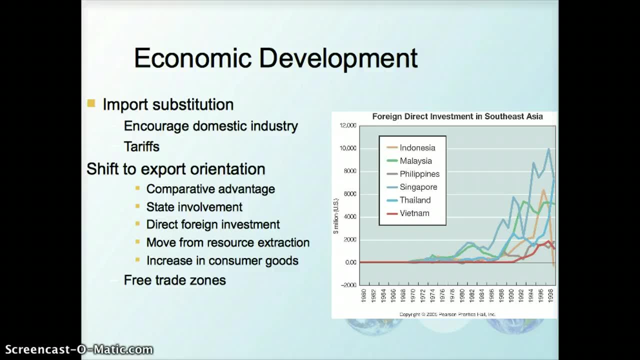 with uh mandalay and rangoon, and vietnam with hanoi and ho chi minh city. if we look at economic development after independence from colonial rule, a lot of these companies engaged in import substitution to try to encourage domestic industry and set up tariffs to protect their industry from competition from other parts of the world. 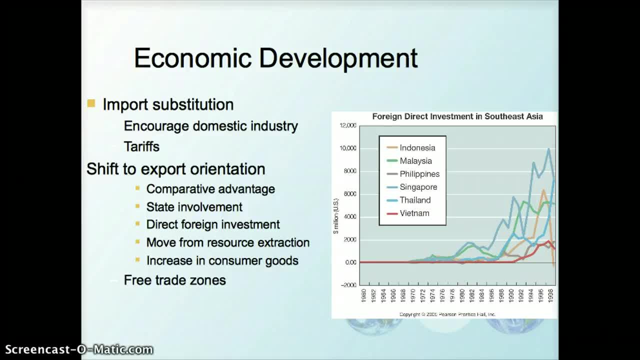 there's been a shift to export oriented production and the search to try to find competitive, comparative advantage things that these parts of the world can produce more efficiently than others similar to East Asia. you have a lot of state involvement in economies and then also foreign direct investment coming in. 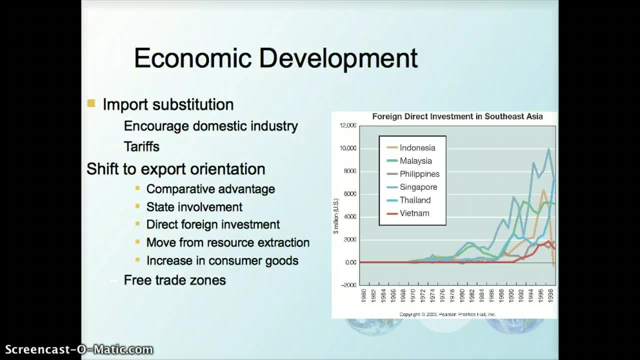 and much of that from other players within Asia. there's been a move to towards our resource extraction and an increase in consumer goods. you see a lot of this new development happening in those free trade zones, somewhat similar to the special economic zones that you saw in China, where companies are given a 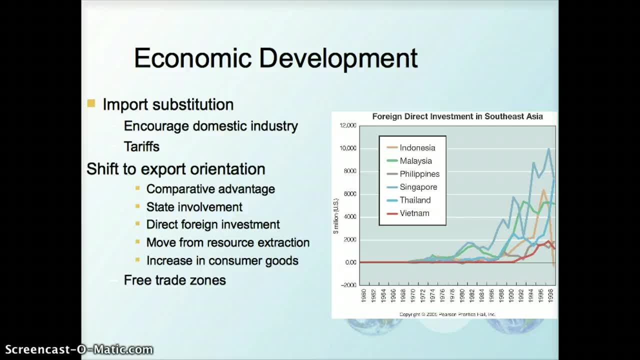 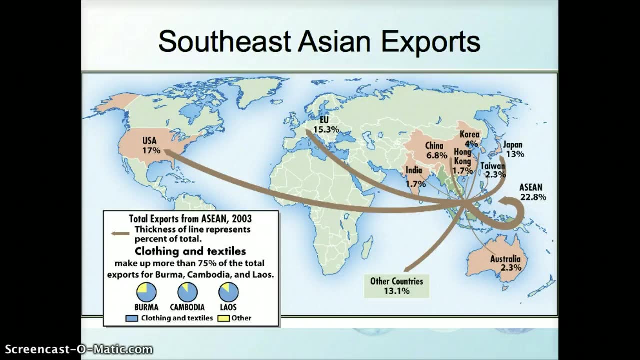 place to come in, set up shop and not have to pay the same sort of trade taxes and tariffs that they would in other parts of the country and be supplied with cheap labor there. if we look at exports, we can see that a lot of the exports in Southeast Asia are based around clothing. 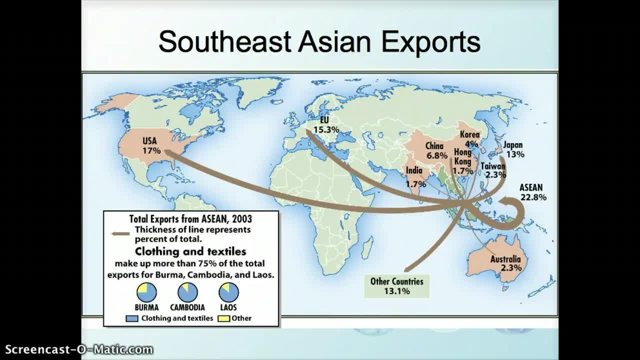 and textiles. so, for example, more than 70%, 75% of the total exports for Burma, Cambodia and Laos, our clothing and textiles. you see a lot of those going into the Asian region, so to places like Japan, a lot to the European Union and a lot to the 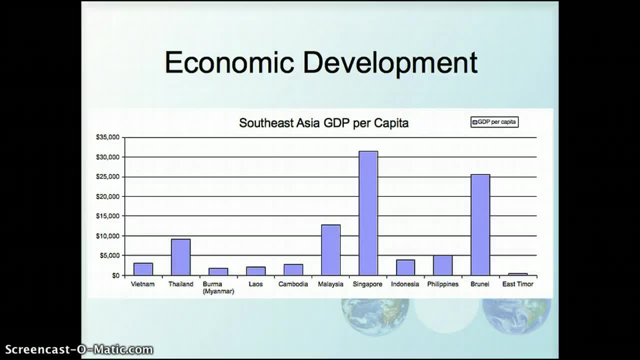 United States as well. If we look at economic development indicators such as GDP in Southeast Asia, we can see that some countries, such as Singapore, Brunei and Malaysia, have a fairly high GDP- Singapore of over $30,000 a year. Other countries are much poorer in terms of GDP per capita: Vietnam, Burma, Laos. 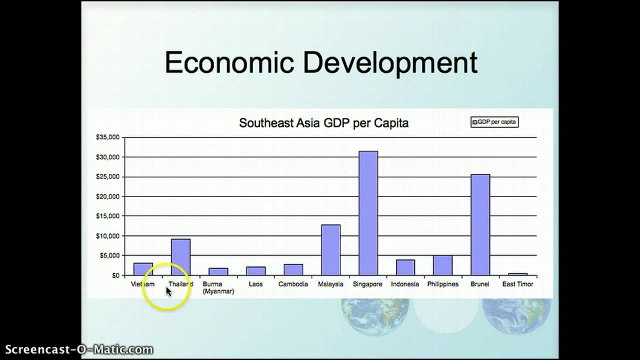 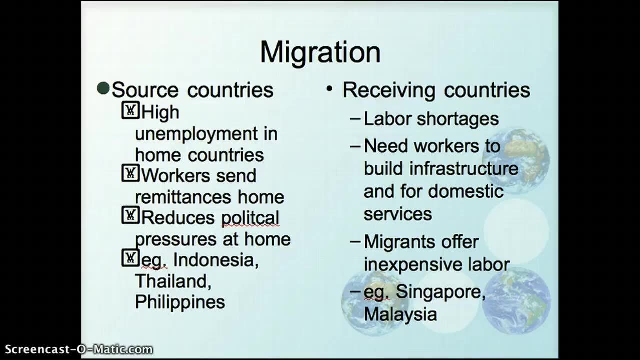 Cambodia, Indonesia and the Philippines. They are particularly poor, with under $5,000 worth of GDP per capita. With that unevenness of development, it's easy to see why migration might be a major factor. within Southeast Asia, Like in other parts of the world, we see the source countries where migrants are. 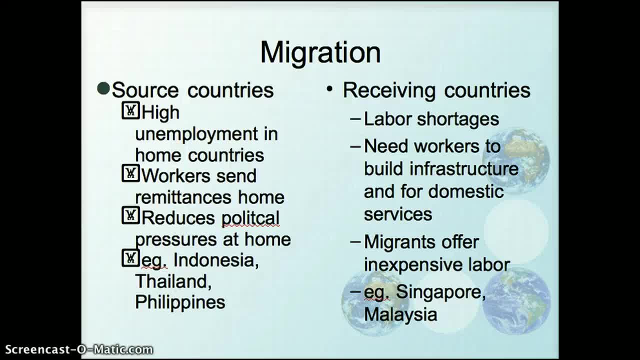 coming from as having high unemployment. Workers want to go work in other countries so they can remittances or money back to their homes and their families. This also helps reduce political pressures at home. You know, there's always that pressure for the government to help people. 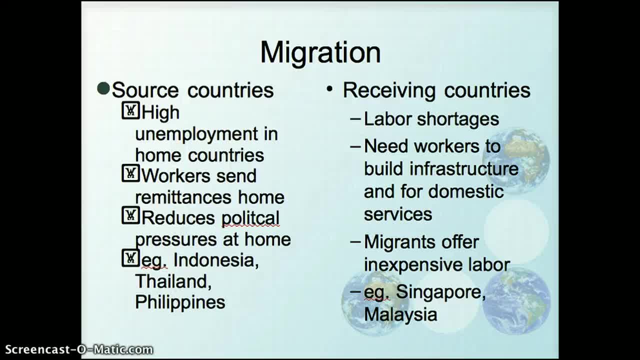 that are struggling to try to find a job, things like that. So it's a major factor in Indonesia, Thailand and the Philippines, and we'll look at that here in a second. Receiving countries are places that have labor shortages, need workers to build infrastructure and for 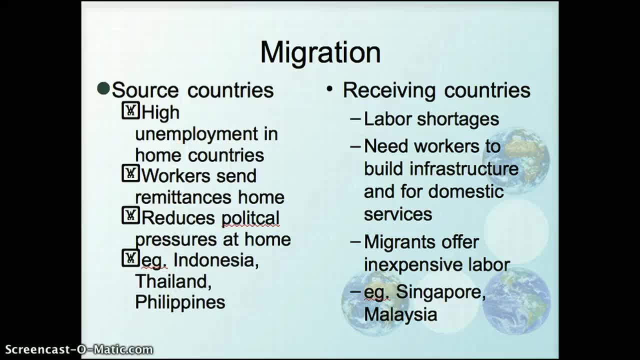 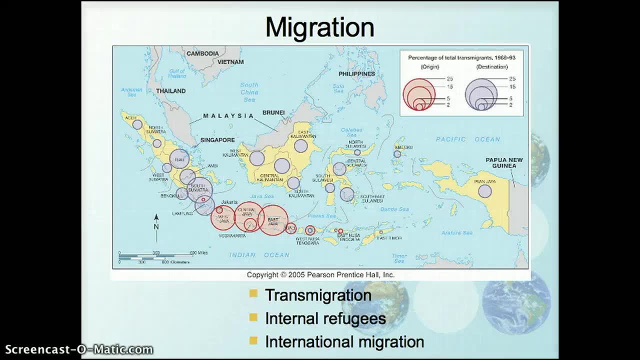 domestic services and migrants are really, you know, very cheap labor often and come into countries with few rights and are easy to exploit. So you see this within places like Singapore and Malaysia. So this looks at migration just within Indonesia. The most populous part of Indonesia is the island where Jakarta is located and you can see that as 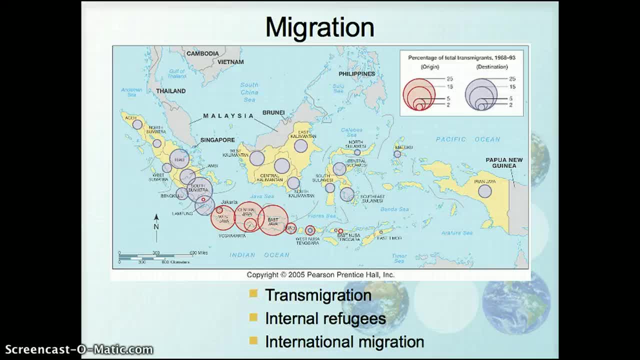 having a lot of these red circles here showing it as a place where you can find a lot of people. So you can see that as having a lot of these red circles here showing it as a place of origin for a lot of migrants. Again, you know the political establishment within. 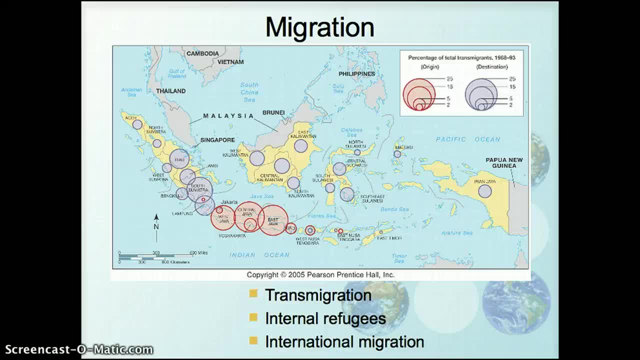 Indonesia if they're unable to find work and employment for people living on its most populous island. they are encouraging folks to move out to other parts of Indonesia where there's less people, to try to sort of mitigate their desire for employment when the country isn't able to provide it. 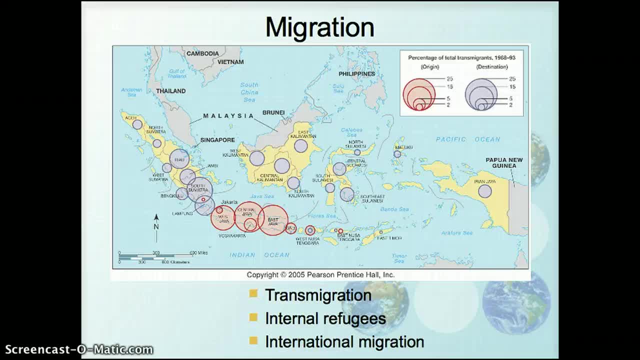 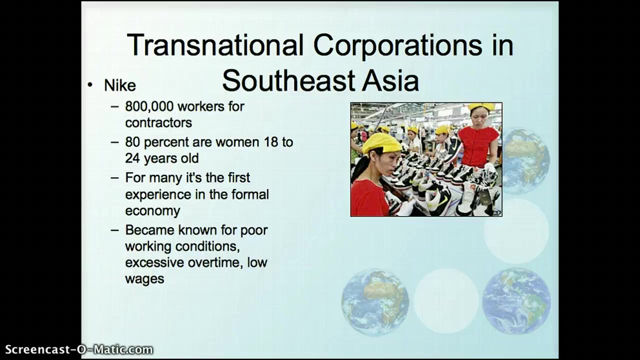 The link to the blue elephant video shows you some examples of migrants, not just from within Southeast Asia, but from other parts of the world, coming into Malaysia to work in transnational corporations' factories. Transnational corporations in Southeast Asia have had a big impact. A lot of them are names of brands that we know, such as Nike, where. 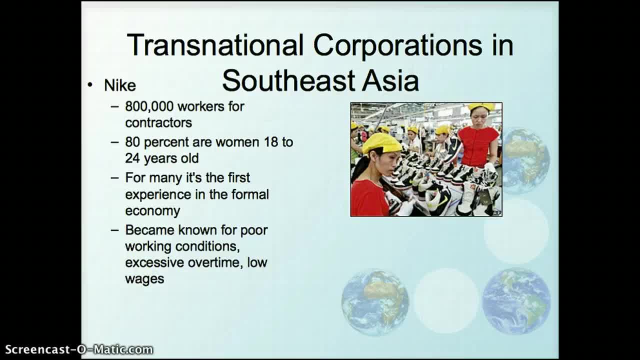 over 800,000 workers work for contractors. Over 80 percent of these are young women that are working in the formal economy for the first time and are well known for things like poor working conditions, excessive overtime and low wages. One of the things that folks 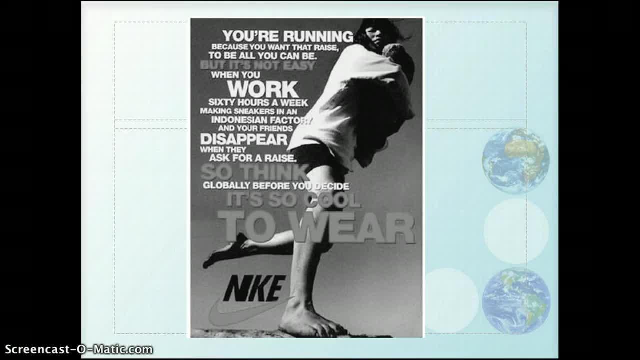 have done to try to combat these concerns about worker exploitation is to try to connect consumers in the developed world with folks that are working in the developing countries. So you see this ad that kind of plays with the symbolism Nike often uses to advertise. It looks at the idea of how those commodities are actually created. So if you take a second, and read this, you'll see how they're trying to use that.